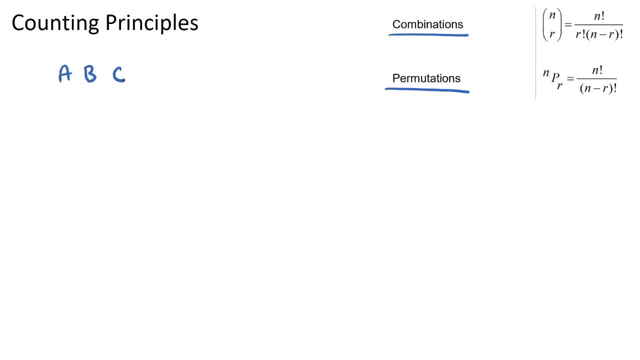 let's use three letters: A, B and C. If I asked you how many ways could these three letters here, A, B and C- be arranged? Well, A, B, C would be one. We could have A, C, B, And then, if I started, 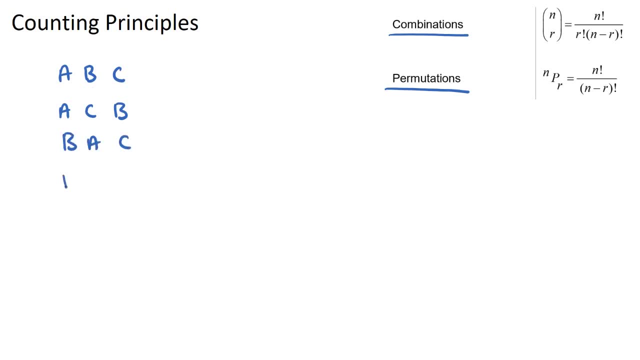 with B, I could have B A C. I could then have B C A, And then, if I start with C, I'll have A B and C B A. So if we were to count these up, there would be six, six ways, and these are: 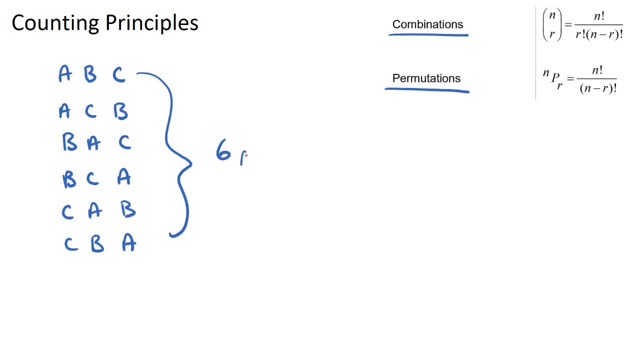 called permutations. So there would be six permutations here, permutations to order these three letters in all of their different ways. Now, what a combination is is a combination is the same as a permutation, except the order doesn't matter. So if I were to say to you how many ways could 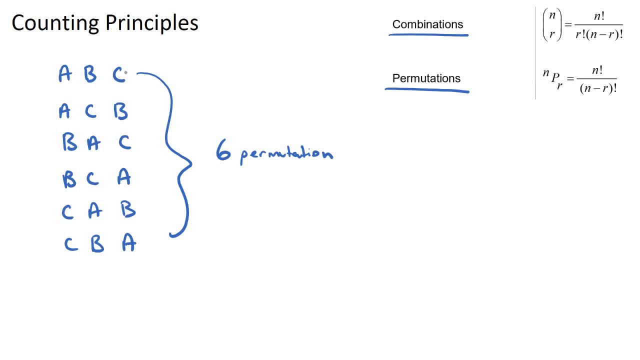 you order A B C, but the order doesn't matter. Well, there's only one way, It's just A B C And A C B, these two here. these are two different permutations, but they're the same. 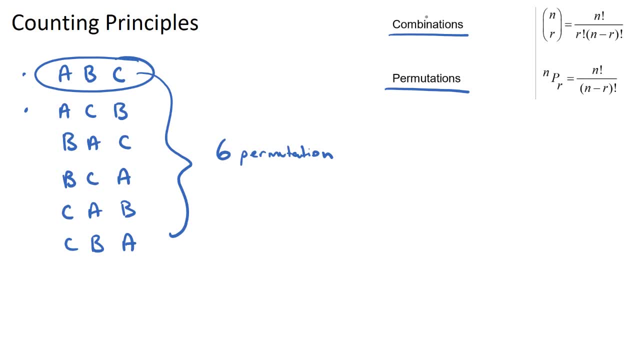 combination. So combination is where the order doesn't matter, Permutation is when the order does matter, So they are different. Now what you may have learned is, if you have three things like A, B, C or three items, the number of permutations is just going to be three. 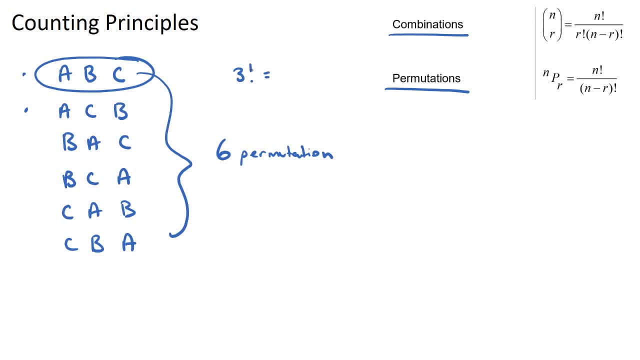 factorial And three. factorial is three with this exclamation mark, and this is just that number multiplied by all of the numbers below it. And three times two times one is equal to six. So if you ever get any question, how do I order? 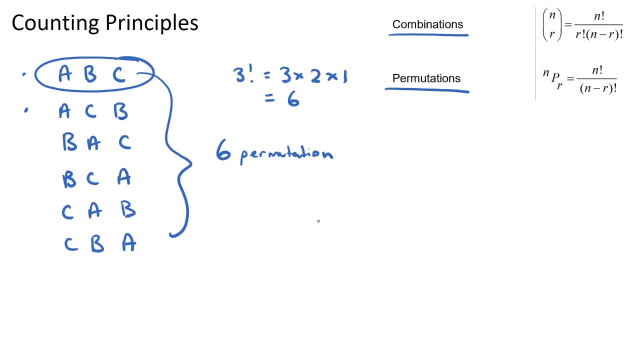 or how many ways can I order 10 different things? It would just be 10 factorial, Or four different things, it would be four factorial, and you just work out how many. that is Now what these questions then do is they get a little bit trickier because they may say, okay, well, if I 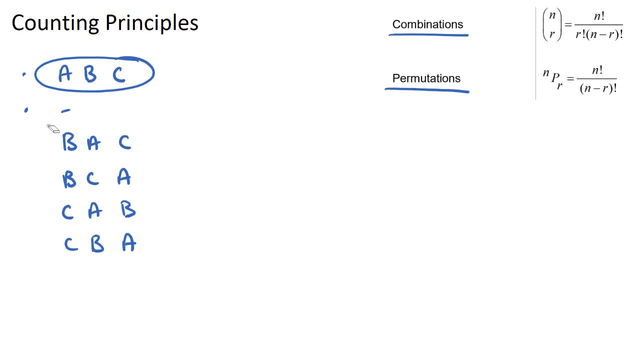 have. let's go back to my three original letters, and I'm going to add another letter, the letter D. And if the question said: well, how many ways could we write A, B, C, D? But we only want to. 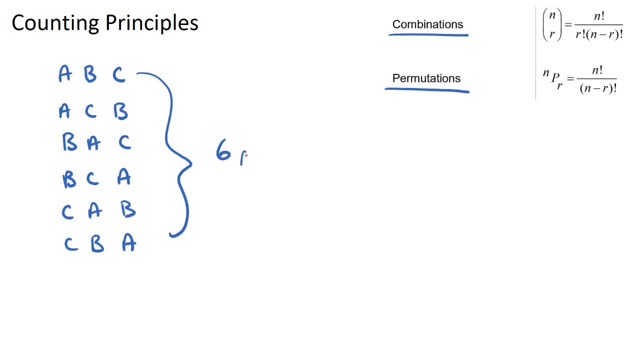 called permutations. So there would be six permutations here, permutations to order these three letters in all of their different ways. Now, what a combination is is a combination is the same as a permutation, except the order doesn't matter. So if I were to say to you how many ways could 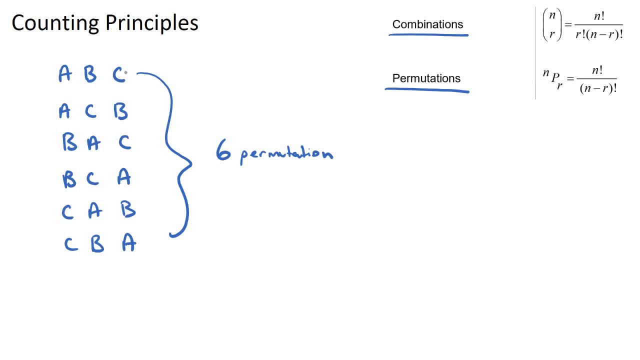 you order A B C, but the order doesn't matter. Well, there's only one way, It's just A B C And A C B, these two here. these are two different permutations, but they're the same. 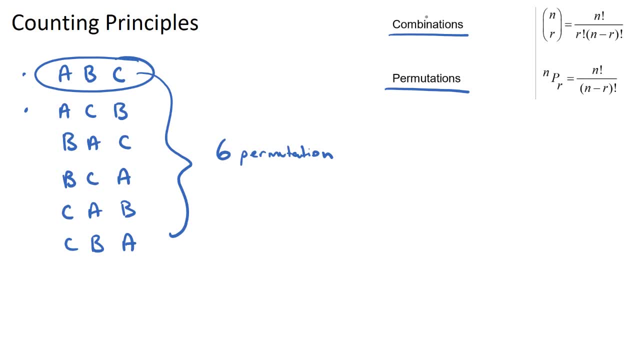 combination. So combination is where the order doesn't matter, Permutation is when the order does matter, So they are different. Now what you may have learned is, if you have three things like A, B, C or three items, the number of permutations is just going to be three. 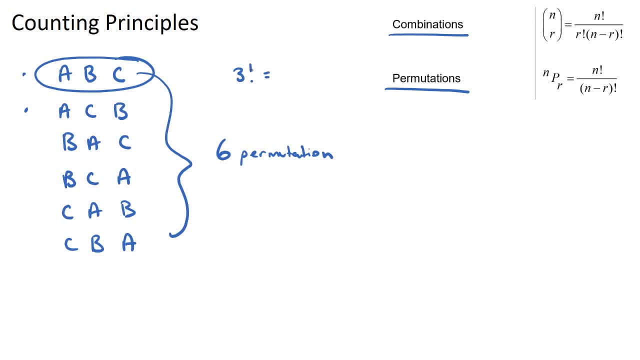 factorial And three. factorial is three with this exclamation mark, and this is just that number multiplied by all of the numbers below it. And three times two times one is equal to six. So if you ever get any question, how do I order? 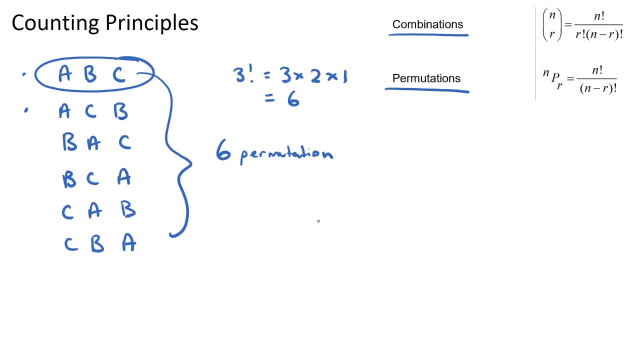 or how many ways can I order 10 different things? It would just be 10 factorial, Or four different things, it would be four factorial, and you just work out how many. that is Now what these questions then do is they get a little bit trickier because they may say, okay, well, if I 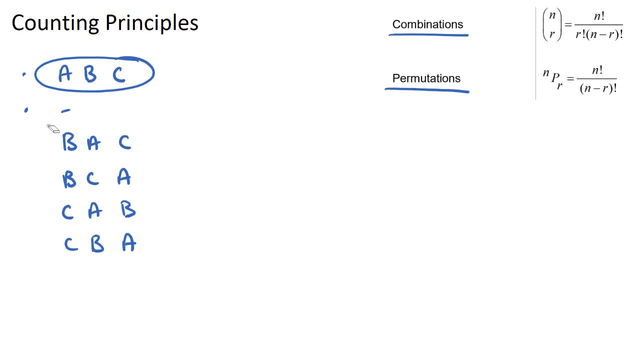 have. let's go back to my three original letters, and I'm going to add another letter, the letter D. And if the question said: well, how many ways could we write A, B, C, D? But we only want to. 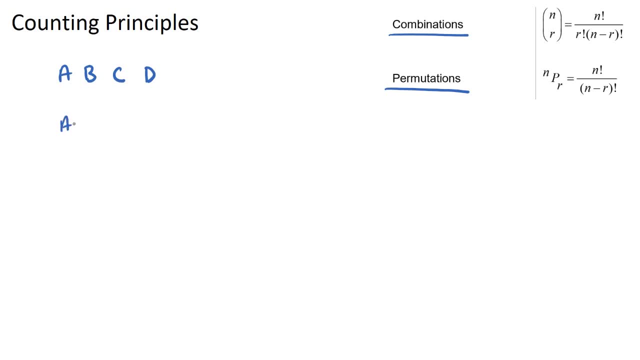 choose two of them. So we could choose A B and then B A and then A C and then C A and then A D and then D A, And you can realize it's going to be quite a lot. And this here was the. 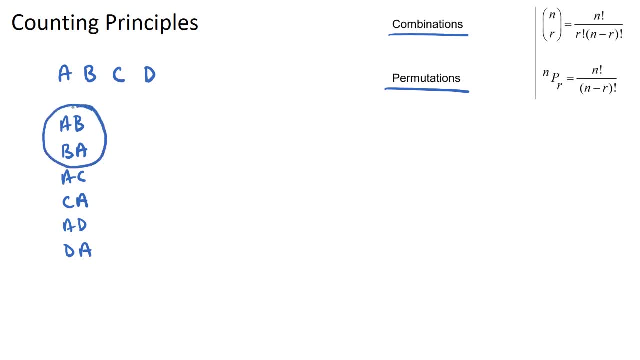 same combination, But they're two different permutations. So that's the key point here: These would be the same combination, but they would be two different permutations. Now, luckily, we have formulas to work out how many there will be. There'll be more than just these ones here. There'll be heaps of. 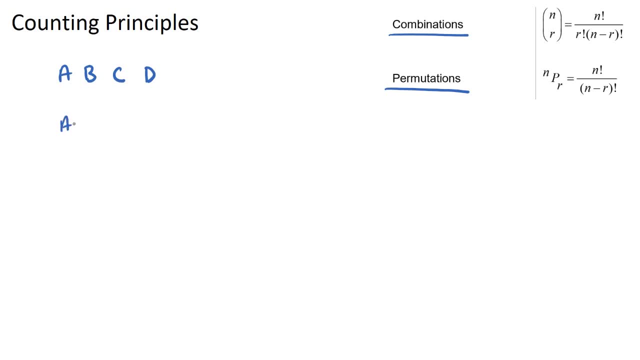 choose two of them. So we could choose A B and then B A and then A C and then C A and then A D and then D A, And you can realize it's going to be quite a lot. And this here was the. 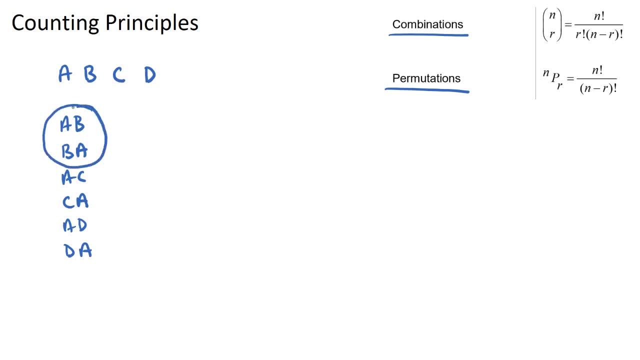 same combination, But they're two different permutations. So that's the key point here: These would be the same combination, but they would be two different permutations. Now, luckily, we have formulas to work out how many there will be. There will be more than just these ones here. There'll be heaps. 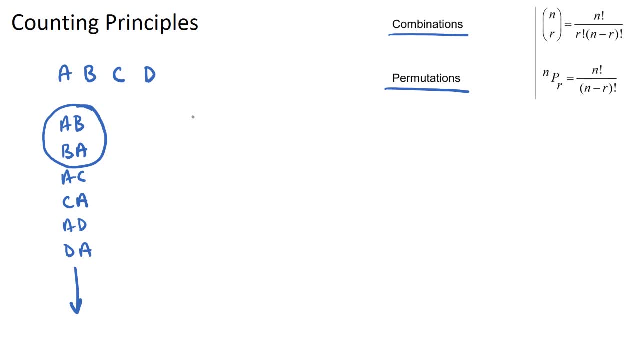 of them And it's these formulas here. The combinations formula for this question would be how many combinations of two from four objects or four letters. So 4C2 would be how many combinations, equations, and the formula for this is just this one up here now. you can see 4c2 written as: 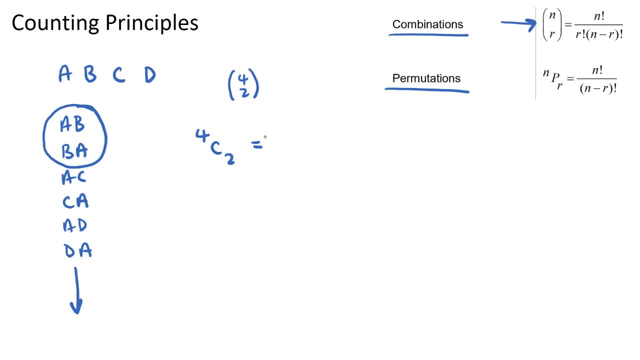 4, 2 on top of each other. that's the same thing. this would just be this top number factorial over the bottom number factorial and then the top number minus the bottom number factorial. so 4 minus 2 is 2 factorial and you can use some algebra techniques to simplify these without. 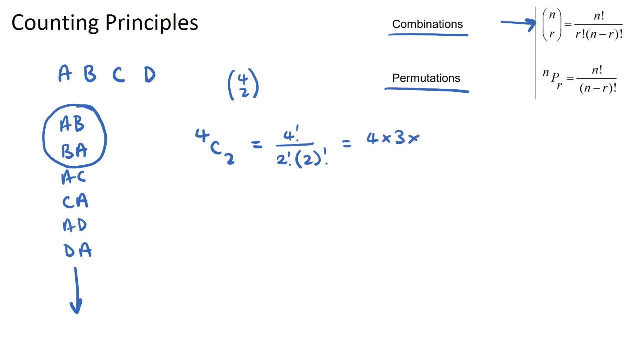 a calculator we can go 4 times, 3 times, 2 times 1, and then you would have 2 times 1 for this, 2 factorial and 2 times 1 and these can cancel out these ones here, and then the 4 can cancel out with. 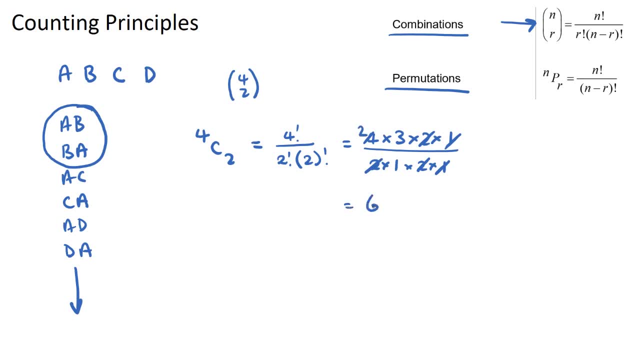 a 2 to be a 2, and we'd get 6 over 1, which is 6. now. this is different to 4p2 permutations. the formula is slightly different. there's no r factorial on the bottom line here, so it would just be 4 factorial over 2, and then you would have 2 times 1, and then you would have 2 times 1. 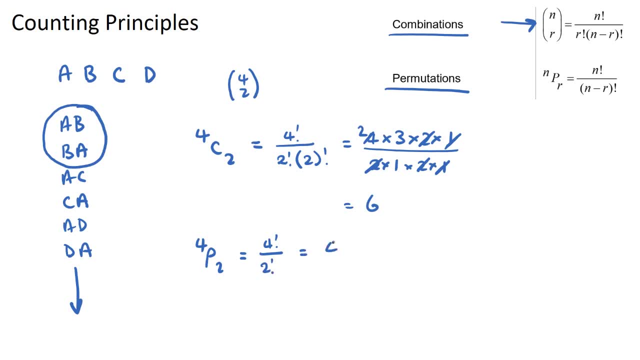 over 2 factorial, which would be 4 times 3 times 2 times 1, over 2 times 1. therefore there will be 12 and hopefully that that kind of makes sense here, because there would be 12 permutations, for our example, but but only 6 combinations. because this 2 becomes 1, these 2 permutations become 1. 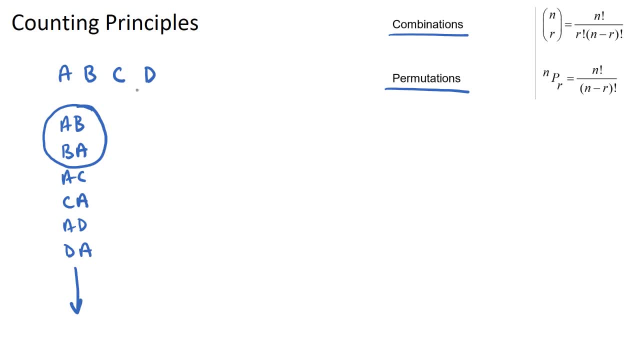 them And it's these formulas here. The combinations formula for this question would be how many combinations of two from four objects or four letters. So 4C2 would be how many combinations, equations, and the formula for this is just this one up here now you can see 4c2 written as: 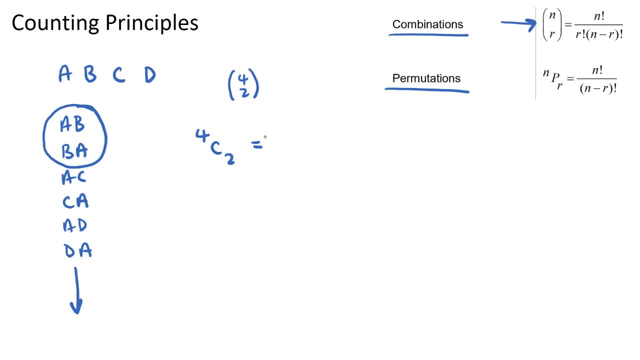 4, 2 on top of each other. that's the same thing. this would just be this top number factorial over the bottom number factorial and then the top number minus the bottom number factorial. so 4 minus 2 is 2 factorial and you can use some algebra techniques to simplify these without. 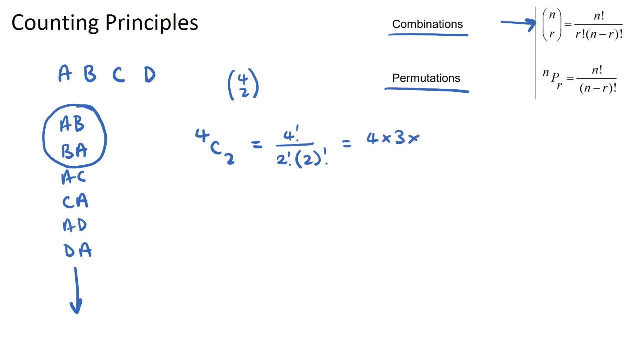 a calculator we can go 4 times, 3 times, 2 times 1, and then you would have 2 times 1 for this, 2 factorial and 2 times 1 and these can cancel out these ones here, and then the 4 can cancel out with. 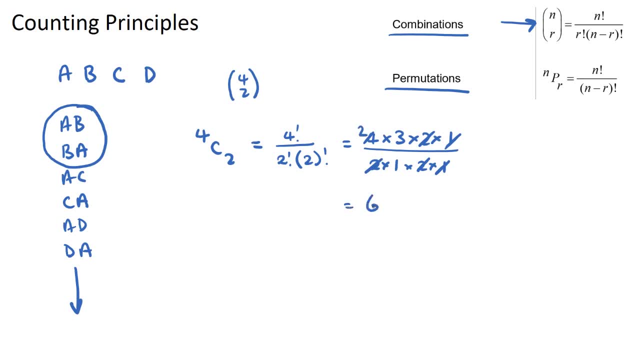 a 2 to be a 2, and we'd get 6 over 1, which is 6. now. this is different to 4p2 permutations. the formula is slightly different. there's no r factorial on the bottom line here, so it would just be 4 factorial over 2, and then you would have 2 times 1, and then you would have 2 times 1. 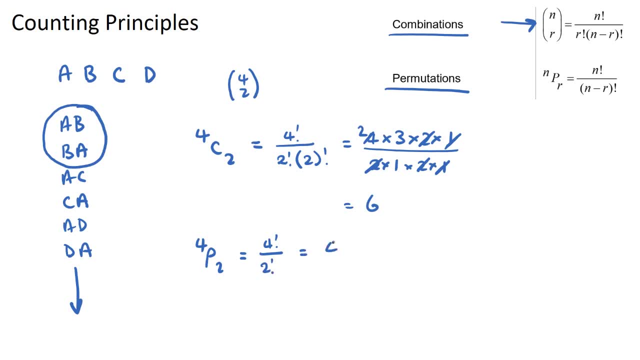 over 2 factorial, which would be 4 times 3 times 2 times 1, over 2 times 1. therefore there will be 12 and hopefully that that kind of makes sense here, because there would be 12 permutations, for our example, but but only 6 combinations. because this 2 becomes 1, these 2 permutations become 1. 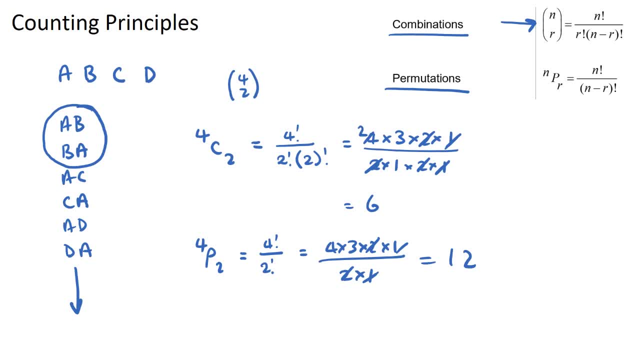 combination. okay, so that's what these, these questions, look like. they do get a little bit trickier when they make sense, and then they do get a little bit trickier when they make sense. they might add multiple elements. they might say: well, if you have 10 options to choose from and 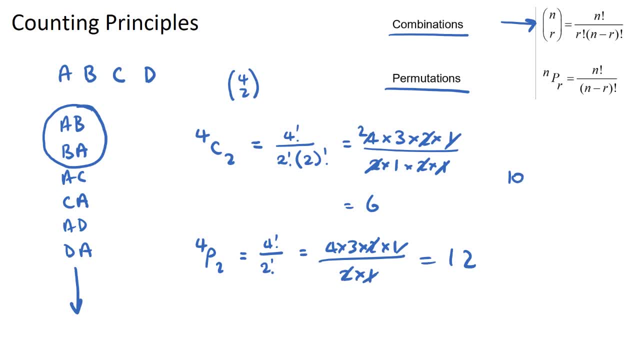 you and you only want to choose 4, and then 8 options and you only want to choose 3, so there might be multiple events happening here. so you'll need to find each of the individual combinations and then maybe multiply them with each other to get the different events. but this is the basic.